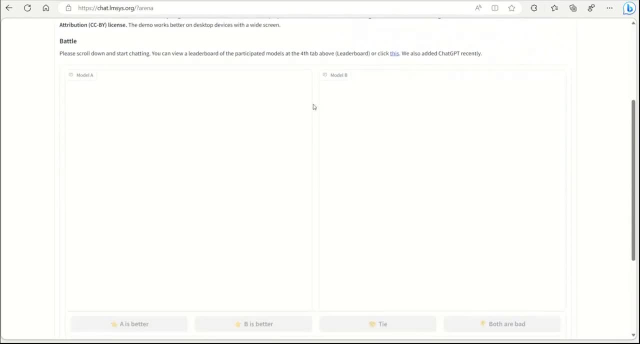 leaderboard in a minute, but I just want to experiment and play around with this blind comparison first. So to do this, we are going to use a very simple prompt. So the first prompt is going to be draft an apology email to a customer who experienced a delay in their order. 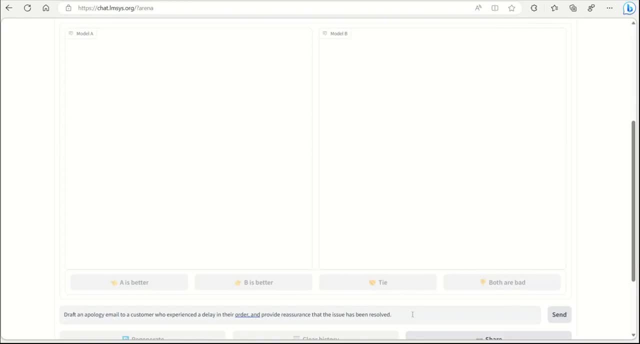 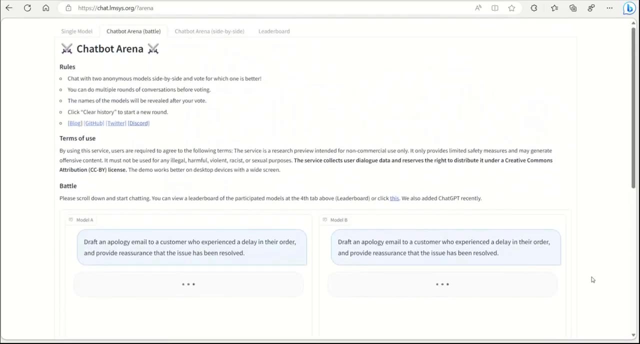 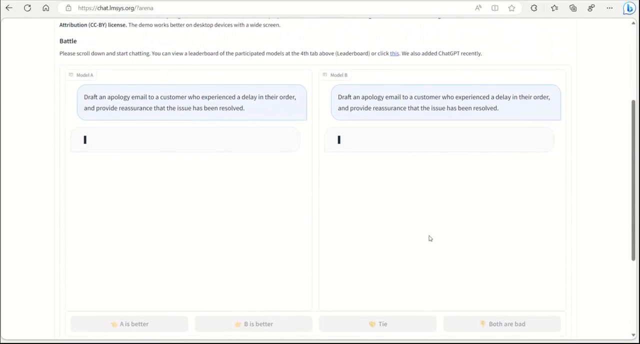 and provide reassurances that the issue has been resolved. Okay, so this is going to be our prompt for the first comparison. So let's send this prompt in and it will randomly pick two models and those models will start generating responses. Now it would be actually interesting if you pause the video and read both responses. 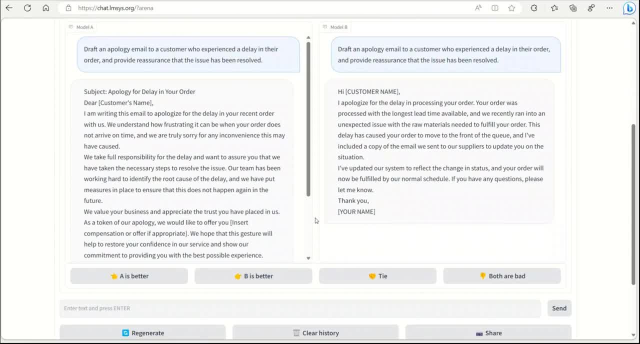 and decide for yourself which model is which you could probably make a guess. So the first one is: I apologize for the delay in processing your order. It's more of a canned response. The thing which I liked it was that it says we recently ran into an unexpected issue with the raw materials. 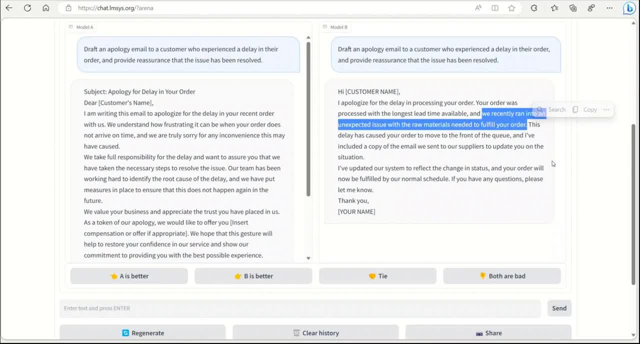 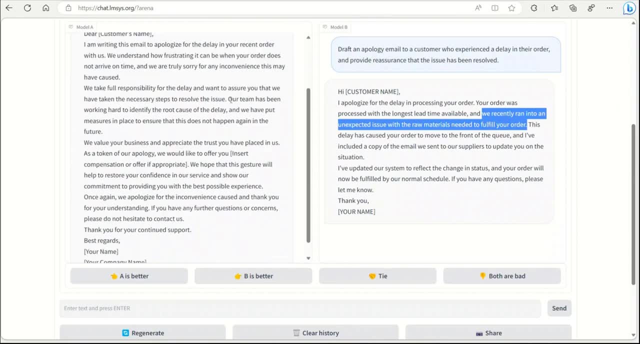 needed to fulfill your order. So it kind of give it and give the customer a cause of the why the delay happened. So this is very nice. Now the second model has a similar response, but it's a lot more detailed. So for example, here it says: our team has been working hard to 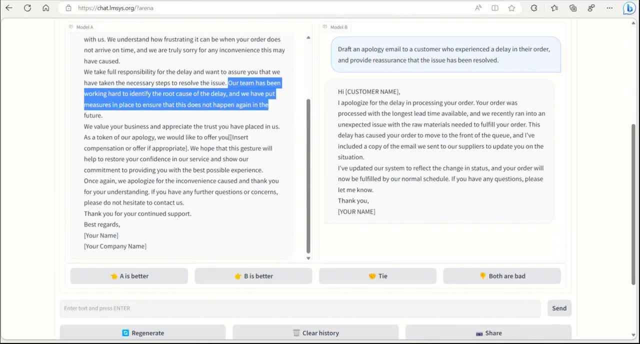 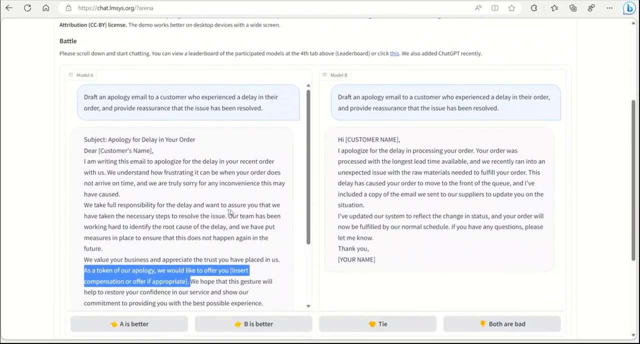 identify the root cause of the delay. And I think which I really liked was that, as a token of our apology, he would like to offer you and then insert, compensation or offer, if appropriate, right. So this is pretty good. I would suspect this is going to be either lacunae. 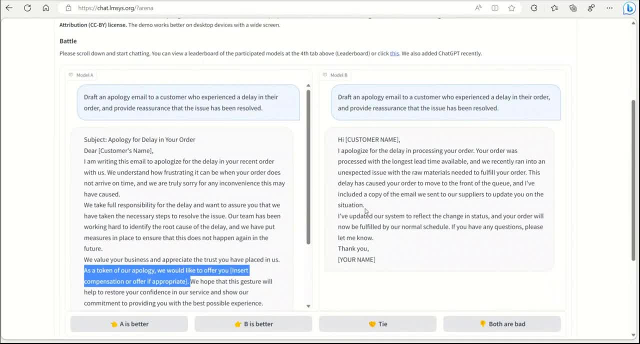 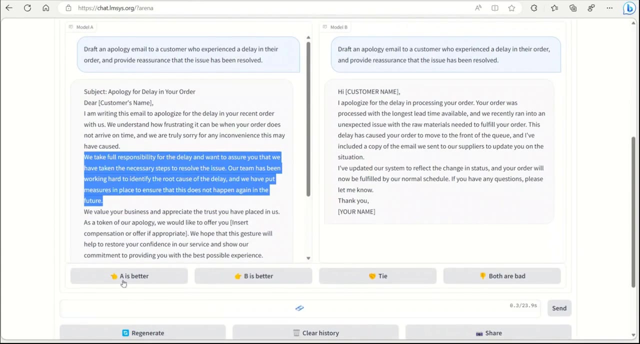 or kawala- And this is probably a smaller model- or even the original lab. they actually have access to GPT for in chat GPT, So sometimes the responses can be coming from them And we don't know ahead of time. But in this case I think model A is better in my opinion. So I'm going. 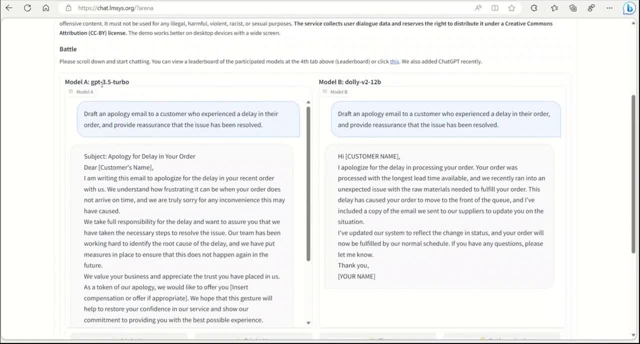 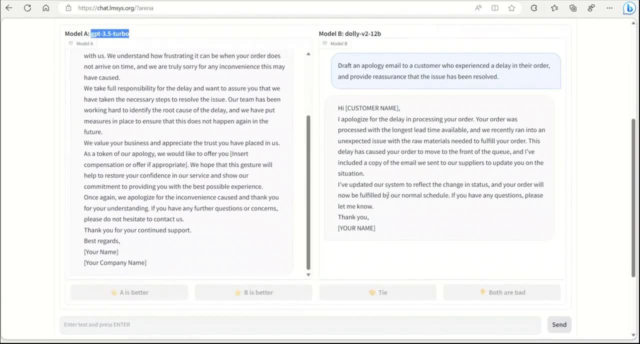 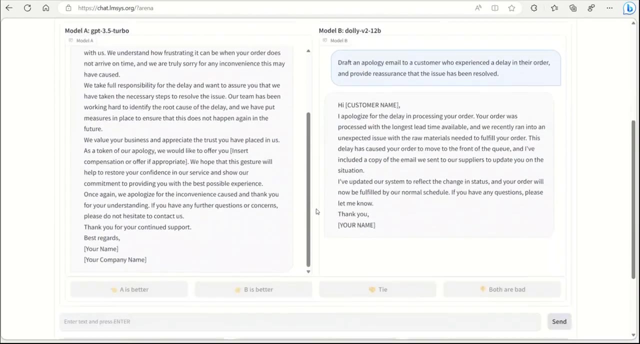 to select model A And then you see that, Oh okay, so actually chat GPT that generated this response And this one is coming from Dolly, Version two. Now, this is a great way of providing feedbacks to the system And your 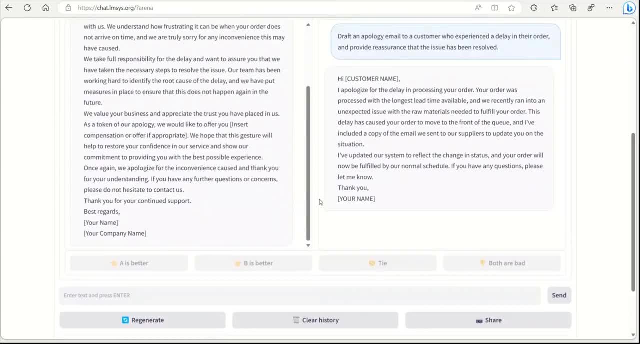 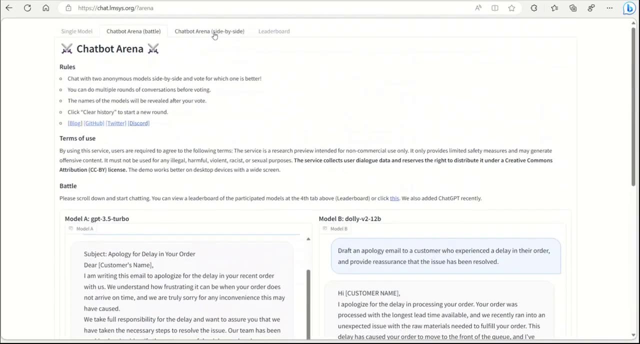 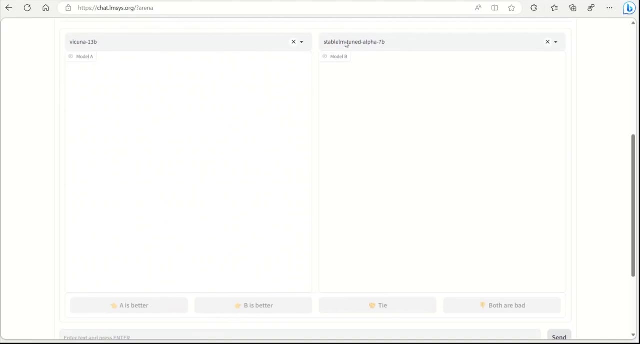 feedbacks are actually used for retraining these models. So it's a great way that you can contribute to the open source efforts. If you want to compare two different specific models together, So you can actually come here and select those. So let's say, I want to compare. lacunae was a stable LM. 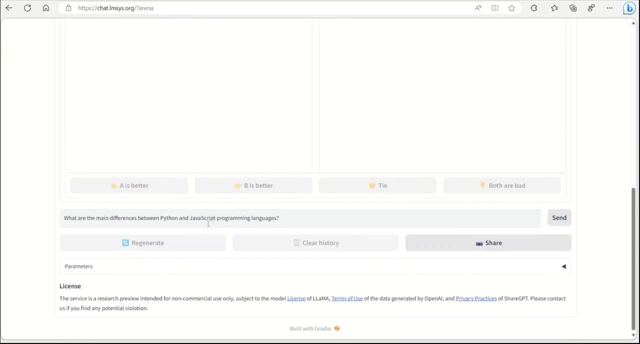 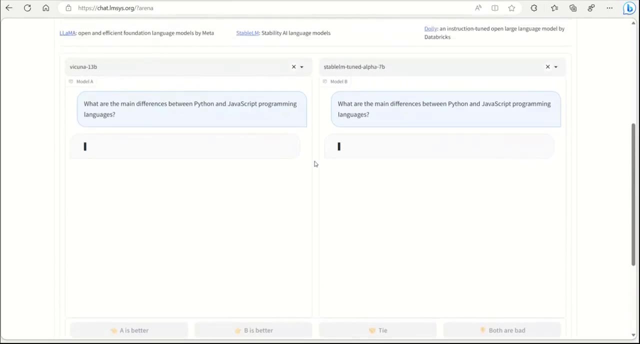 And my prompt in this case is: what are the main differences between Python and Java Script programming languages? So, based on my experience, I would expect lacunae to be better, But let's see. both of them actually came up with a very similar response. So 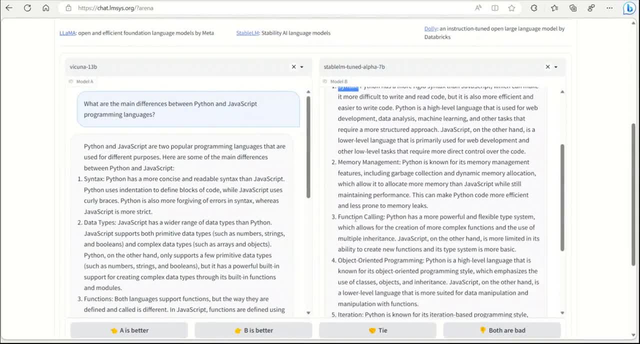 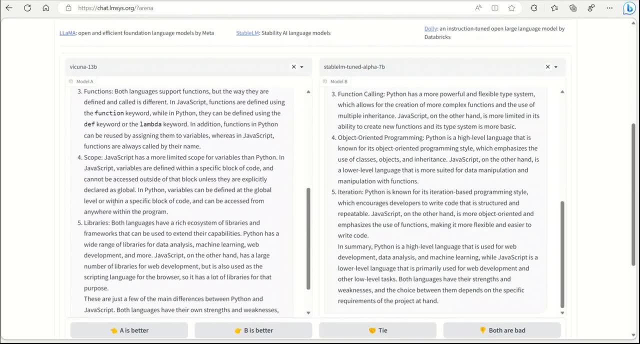 let's say they compare it in terms of syntax memory management function of calling object oriented programming, iteration, And in this case it's syntax- data type functions, scope, libraries, And so I think these are similar responses or similar comparison, But I really 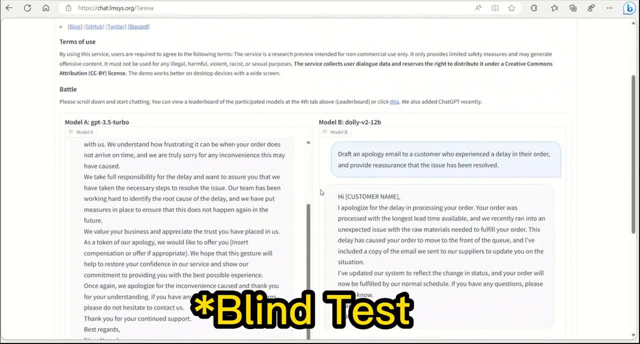 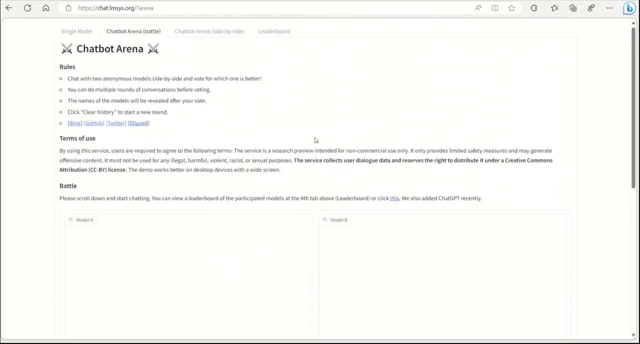 really like this comparison- Because you could be actually really surprised based on the results- is sometimes we think that the smaller models are not really powerful, But what I have seen is- and my responses- sometimes a smaller model can outperform the larger models. Now let's look at the leaderboard. 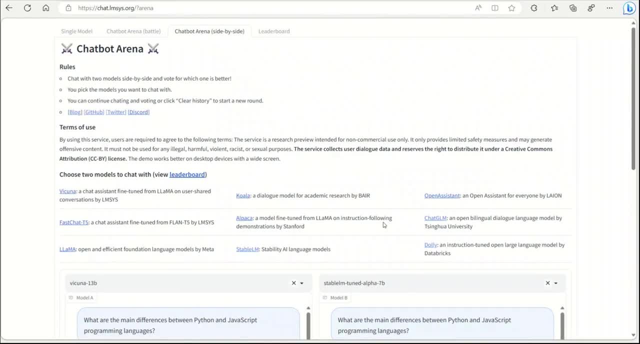 But before then let's see what the community thinks. So maybe order them on the based on what your opinion is. which one are the five at the top? let's say three or five? it would be interesting to see that in the comment section below. if you like to do that, pause the video and maybe post a comment. 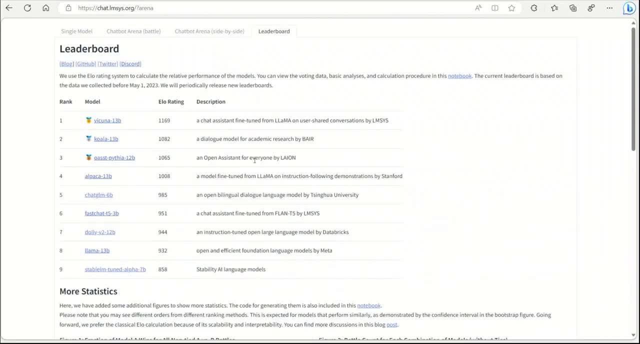 all right. so, based on all the uh, human feedback, here is what people think, right. so this is the great thing about their method: that they are evaluating it on the human responses rather than on some benchmarks. now, keep in mind that the leaderboards board is based on the data that 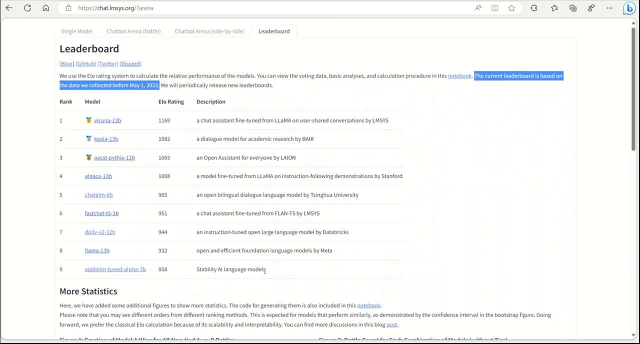 have collected before may 1st. right, so it could change actually, but overall wakonia seems to be the most like model, followed by koala, and then open assistant and alpaca, then chat glm and fast chat dolly. version 2.7- the real world感じ- is actually on a much lower uh rank than i would have suspected and similar to 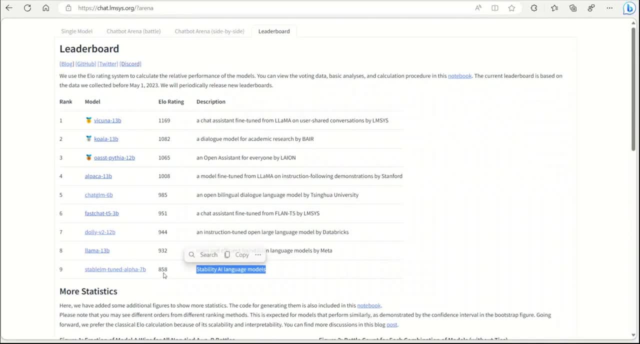 uh, similar is the case with stable lm, but i think stable lm was just released, so maybe that's the case. uh, the most surprise, surprising part for me was, uh, this fast chat, which is a flan t5 model that is fine-tuned, uh, to be like a chat assistant. now, this is the smallest of the models, so it's. 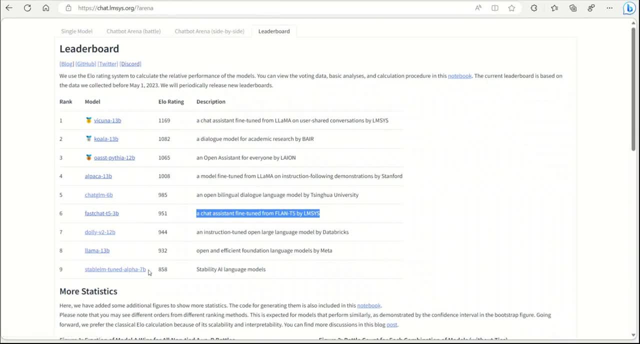 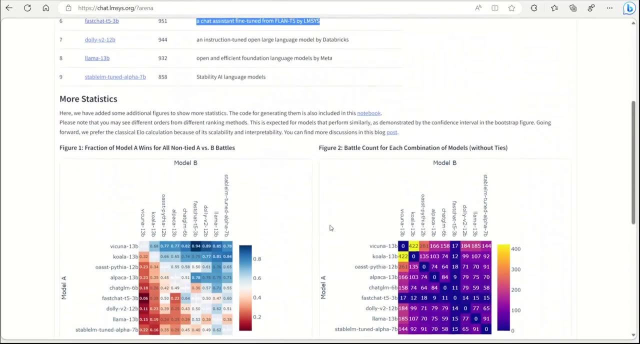 just 13 billion parameter compared to, let's say, 300 million parameters. so i think it's around the 13 or 12 billion parameter, but it's surprisingly uh, doing well compared to the other models. now they have provided a really comprehensive statistical comparison. so let's say: 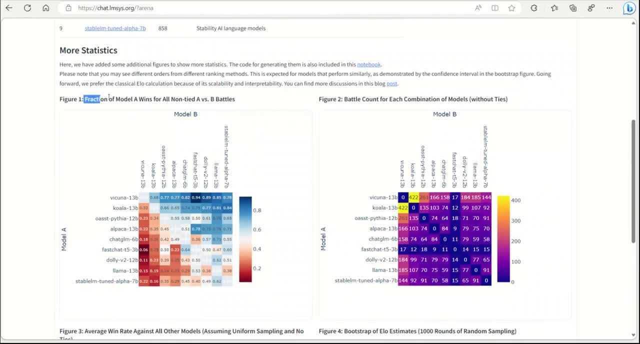 uh, here are a few plots if you guys are interested in. so the first one is: fraction of model a wins for all and non-tied a versus b battles, right? so let's say in this case, uh, wakunya versus the rest of the models, uh, so it's like, if there is a one-to-one comparison, so wakunya was able to beat. 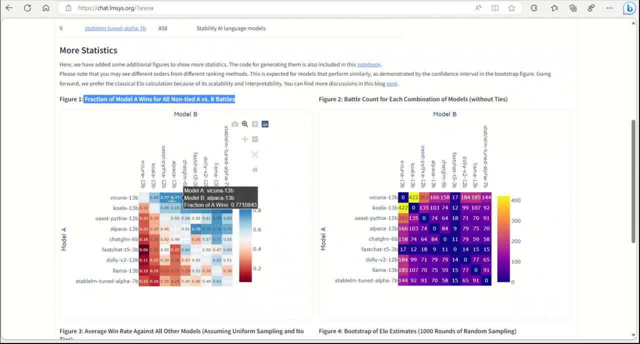 a koala almost 69 percent of the time, 68 percent to be exact. then uh wakunya versus open assistant. so wakunya won around uh 77 percent of the time. right, so you can look at these results and here's a better count for each combination of the model. so this means that how many times different models? 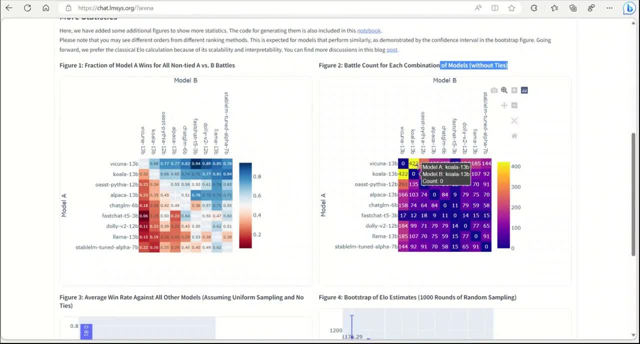 were compared. so let's say wakunya versus uh koala. it was compared 422 times. now, based on these results, you can see that the fast chat t5 model as well as the stable lm models- these are not compared a lot with the rest of. 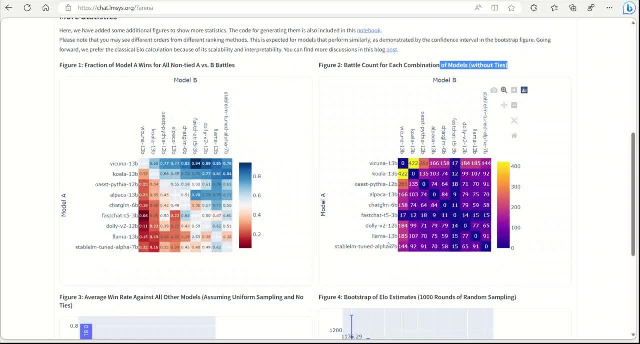 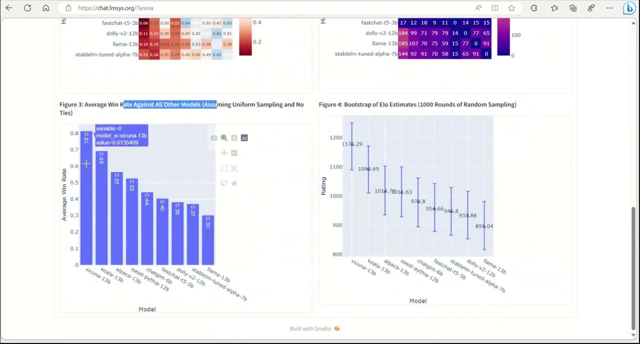 the models, so that could be a reason for stable them not being like high up in the rank. now, if you take average win rate against all other models, so not just one-to-one comparison, then wakunya versus open assistant is the overall winner, and this is probably expected. then there's koala alpaca. 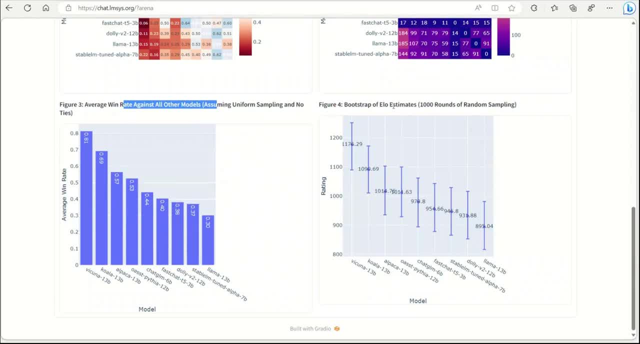 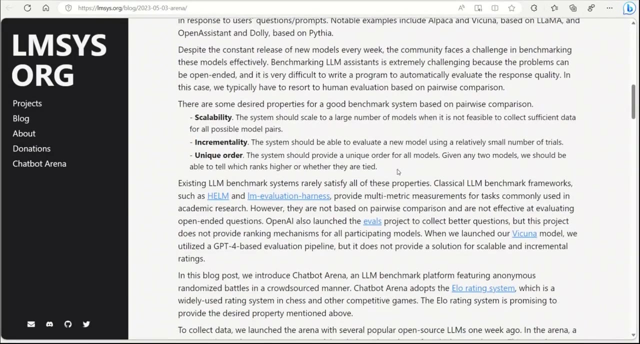 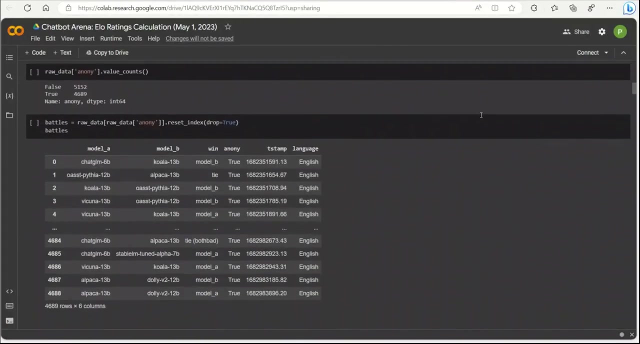 and open assistant. similarly, they provide something called elo scores or estimates, which measure the relative performance of different models, and even on that, wakunya is the top model. they actually have a very comprehensive description based on their methodology, uh, to explain it, and they have even provided a google collab notebook with all the